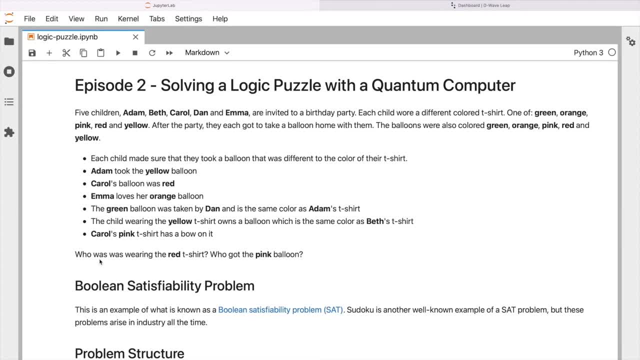 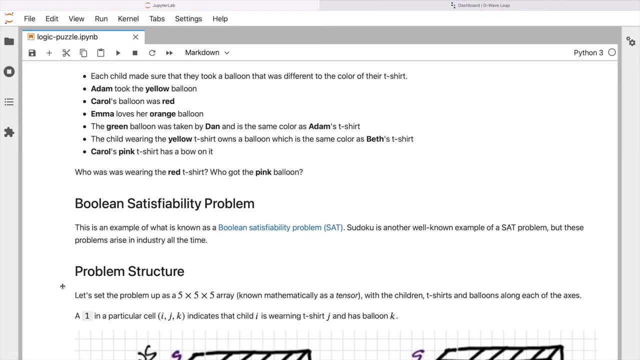 You could solve it with pen and paper, And indeed that's how this puzzle was designed to be solved, But it introduces a lot of the core ideas that we're going to explore around solving optimization problems and constraint problems with a quantum computer. So this is an example of what's known as a Boolean satisfiability problem or a SAT problem. 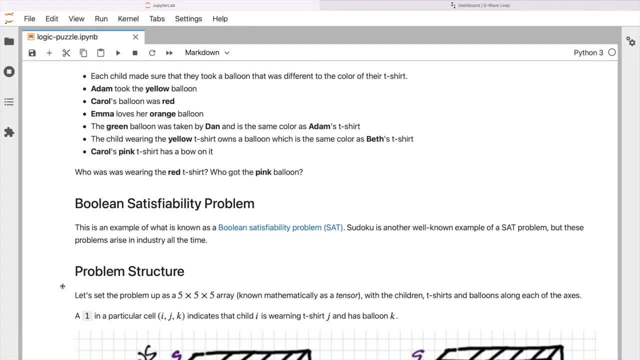 And other well-known examples that you may be familiar with include Sudoku, if you're a puzzle fan, But in fact these arise all the time in industry. They're used to solve scheduling problems and many other types of problems, So very, very applicable and certainly much more difficult than the one we have here. 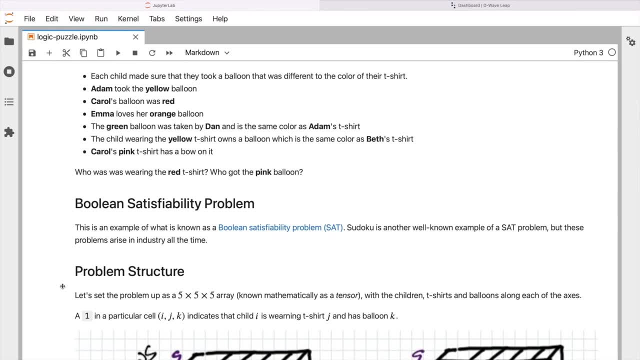 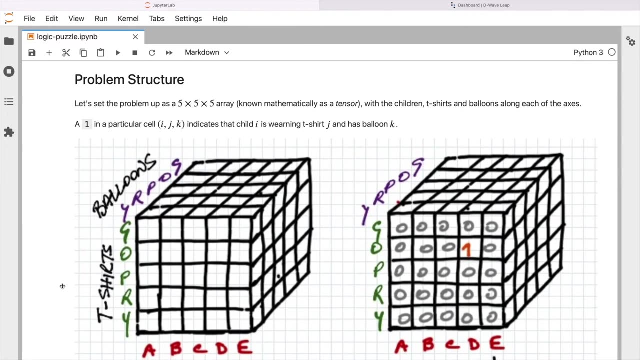 So with all problems, usually the first place to start is to figure out: well, how do we structure the problem in a way that we can actually attack it with a computer? So let's go ahead and consider that. So here we're going to set the problem up as a five by five by five array. 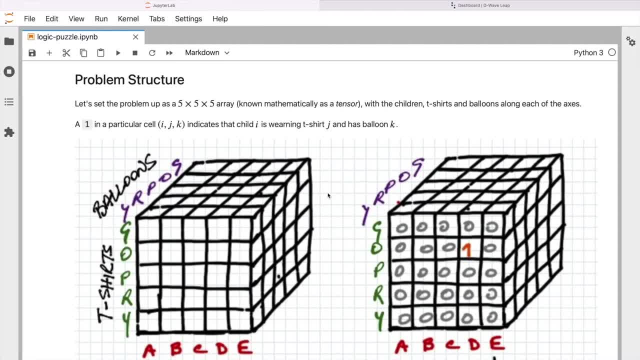 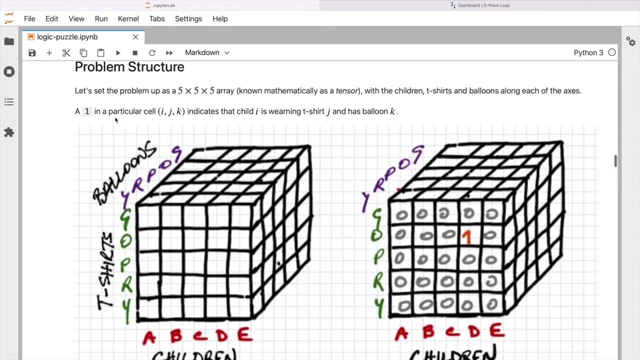 This is known in mathematics as a tensor. And along the axes of this array. we're going to put the children on one axis, the t-shirts, the colors of the t-shirts and the colors of the balloon along that axis. And so here, what we're going to say is that a one in a particular cell, i j k. 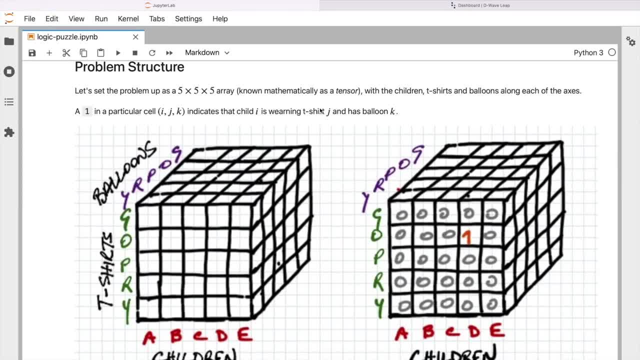 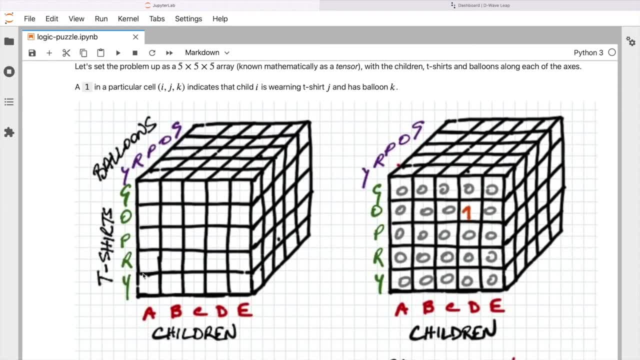 indicates that child i is wearing t-shirt j and has balloon k. So if we look at my poorly drawn diagrams here, for example, this looks a little bit like a kind of a five wide Rubik's cube, But the idea here is that we're putting children along one axis. 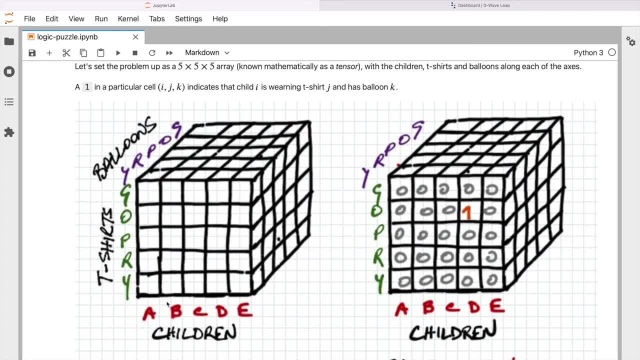 So child Adam, Beth, Carl, Dan and Emma, A, B, C, D, E. And then we have children. We have our t-shirts along another axis- green, orange, pink, red and yellow- and our balloons along a third axis- also green, orange, pink, red, yellow. 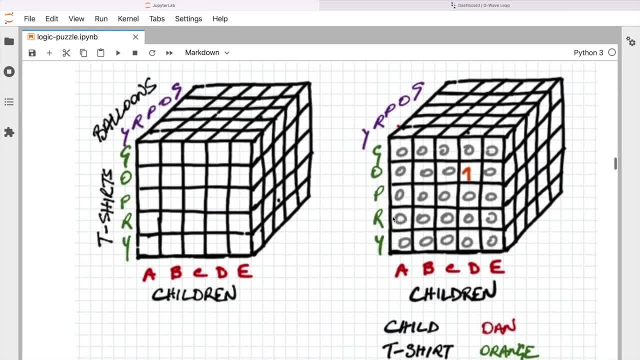 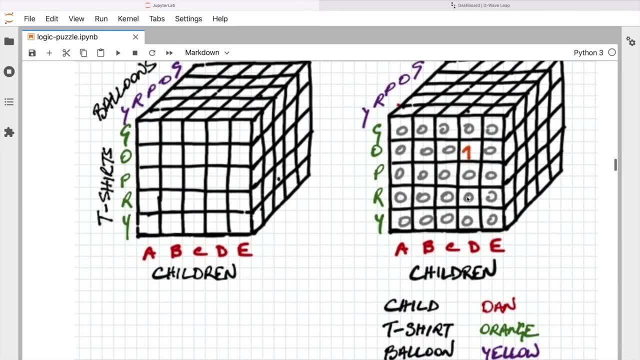 And then we, if we look at the right here, we can see that we have a particular assignment. We've put a one in this entry in the array and zeros everywhere else. So the one tells us that in this particular assignment, child Dan has the orange. 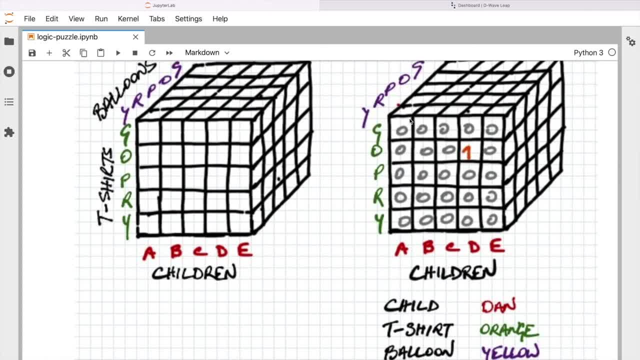 t-shirt and the yellow balloon. Now we don't know yet whether that's a valid assignment, Whether that will help us to solve the problem, But that's at least how to interpret, how we're going to represent potential solutions or candidate solutions. So that's it for this episode.